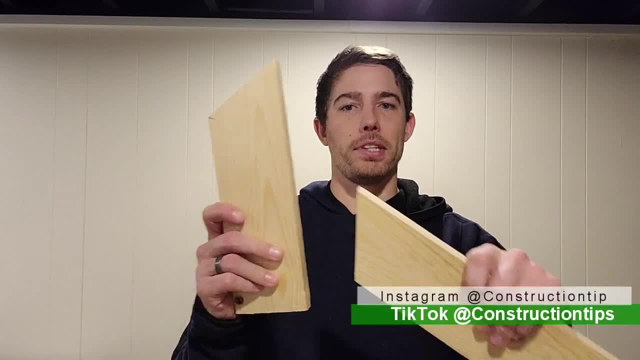 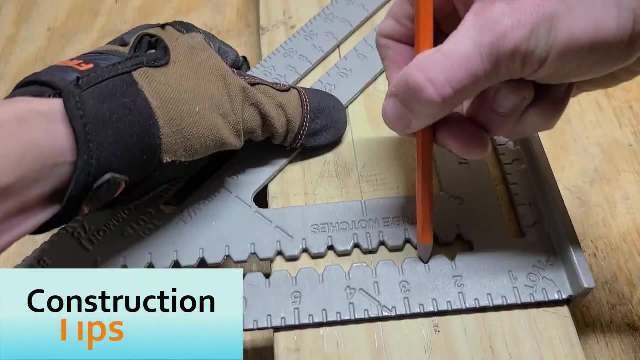 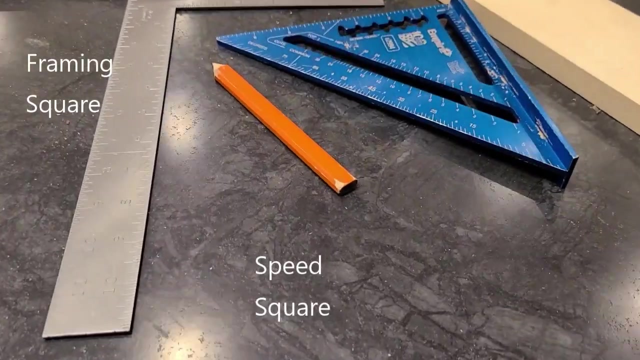 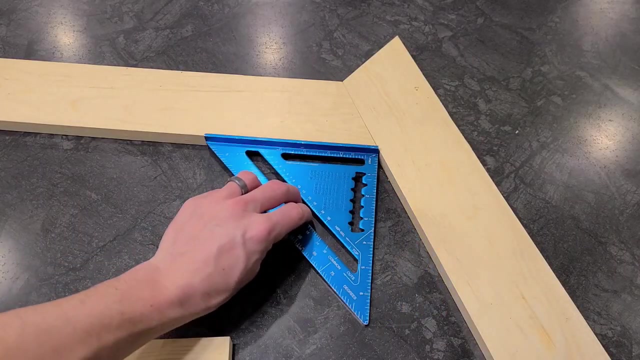 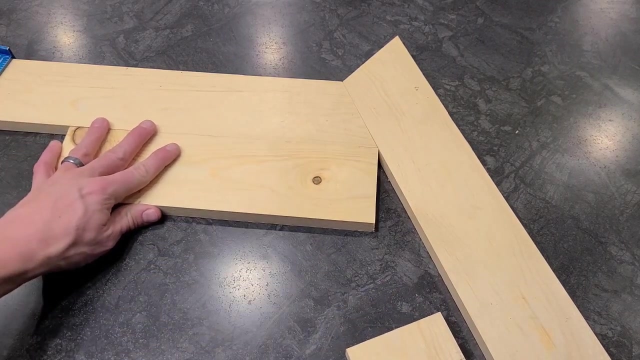 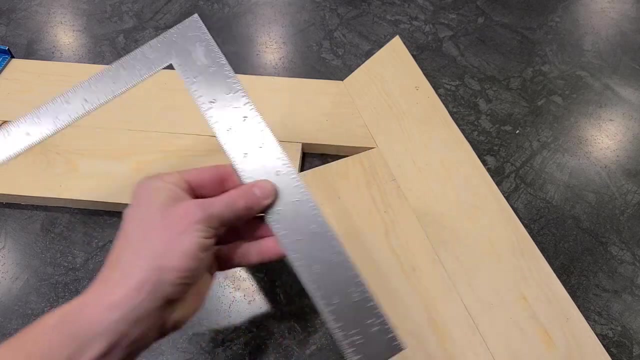 Hey, what's up everybody? Sam, with Construction Tips. Today, I'm going to show you how to find angles like this without an angle finder. So, first of all, let's find angles with the angle finder. I'm going to show you the best angle finder. 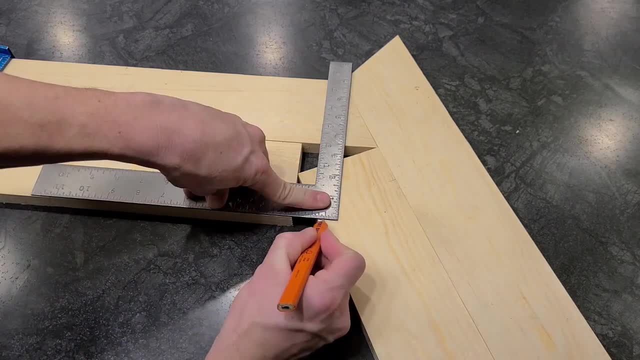 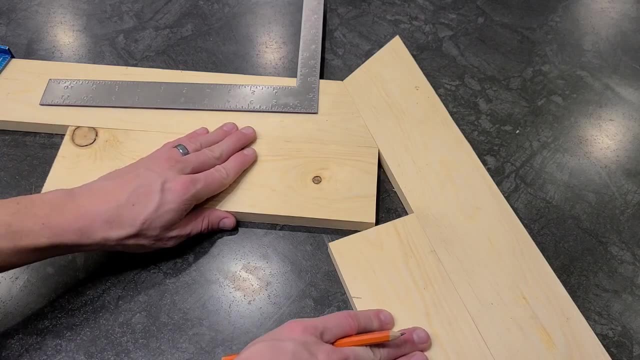 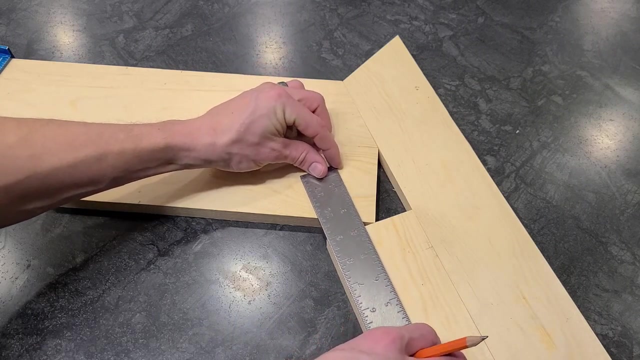 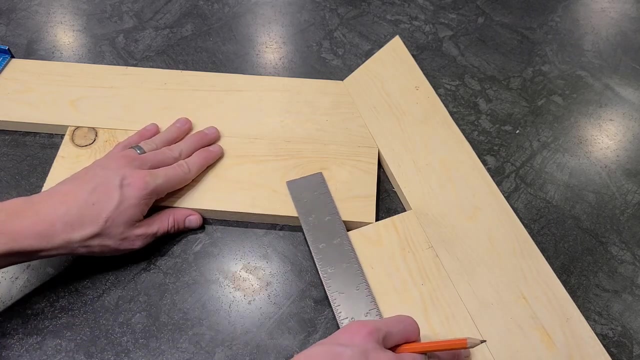 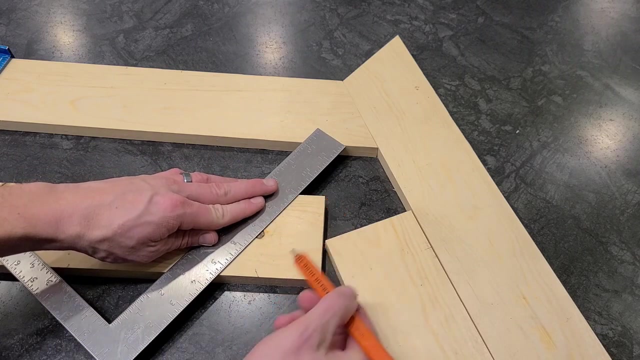 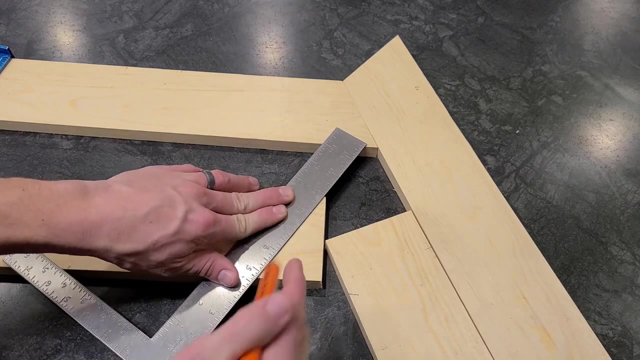 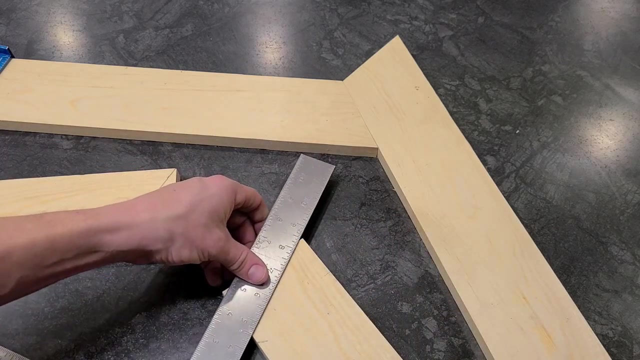 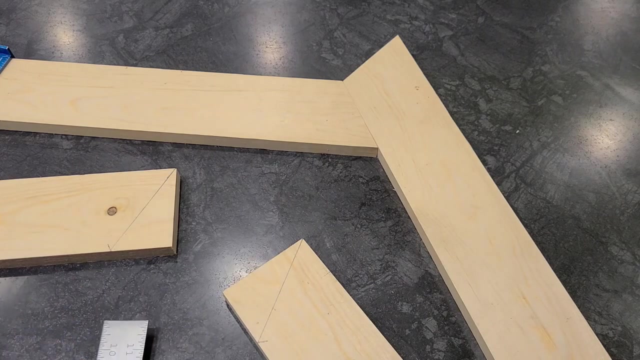 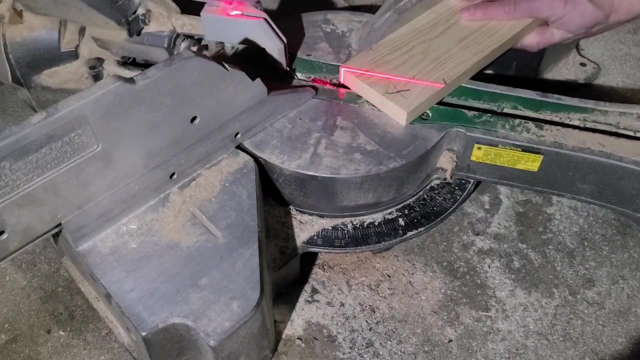 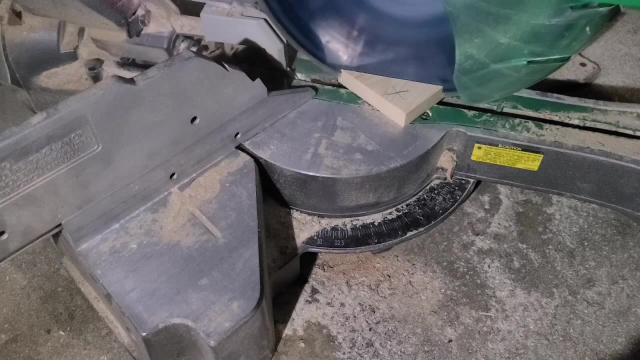 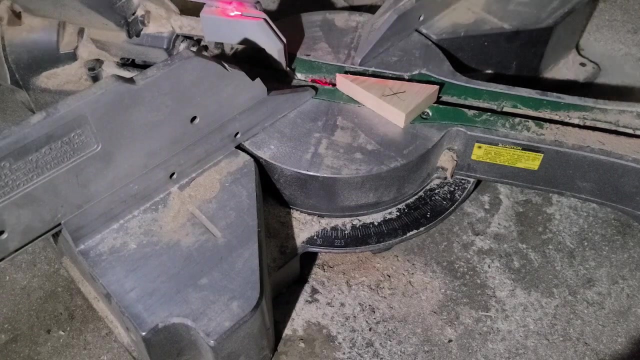 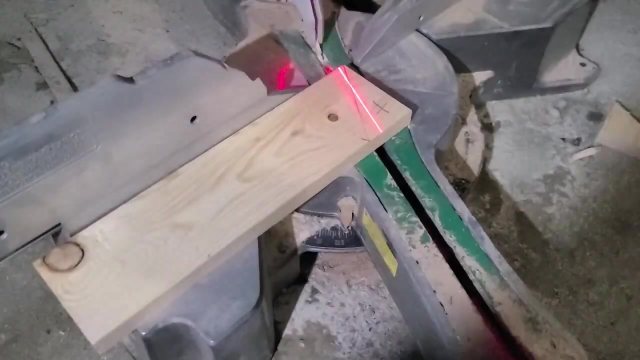 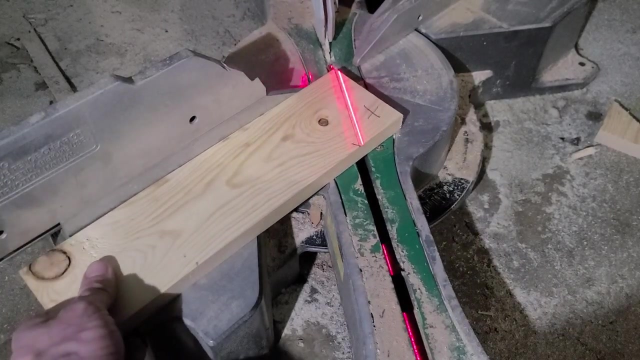 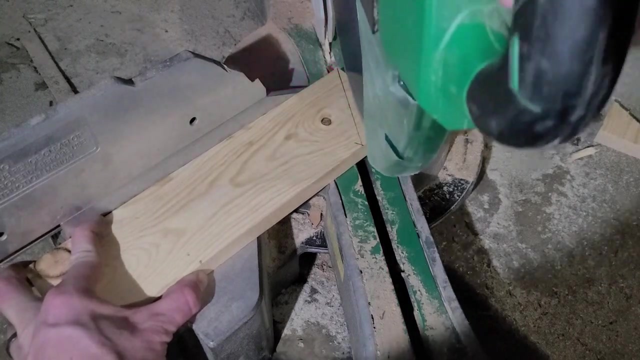 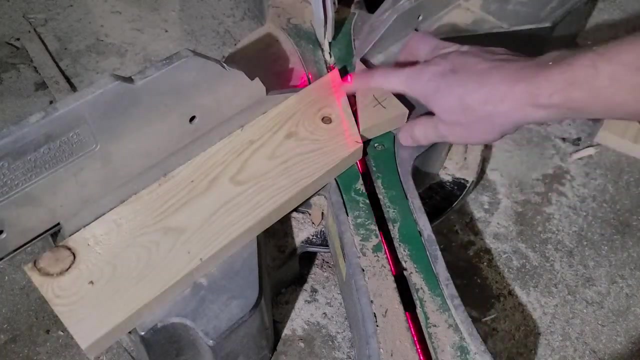 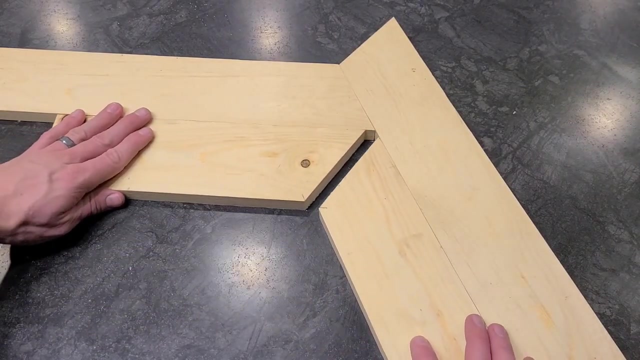 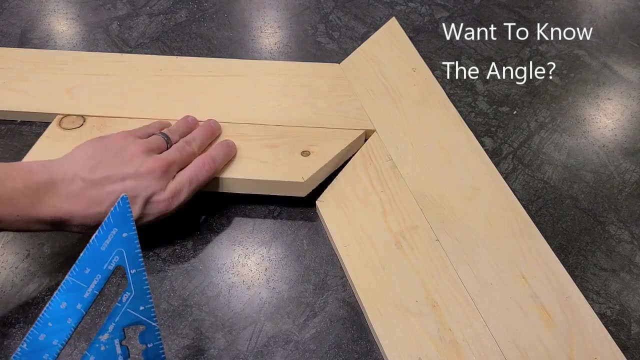 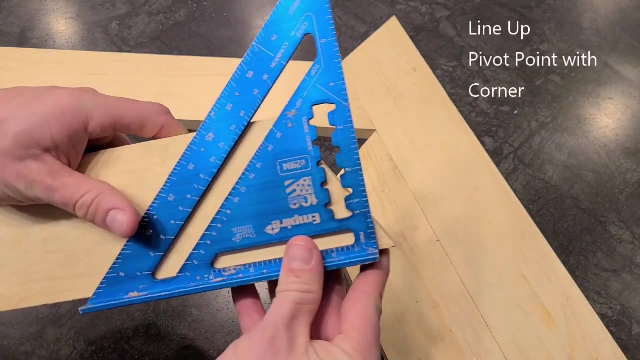